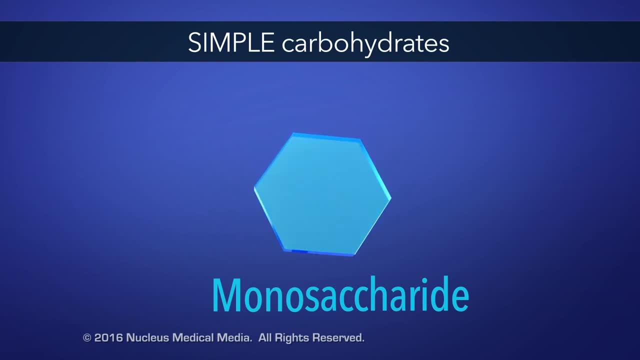 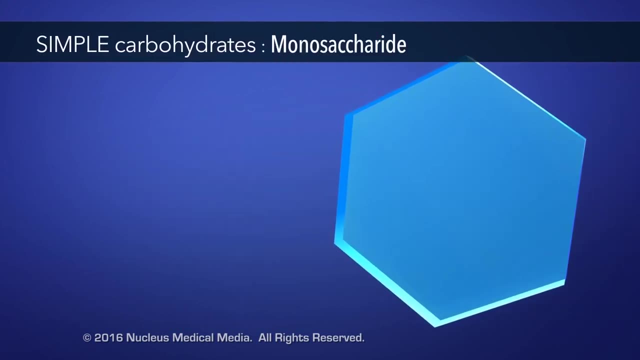 called a monosaccharide, or two sugar molecules called a disaccharide. An example of a monosaccharide is the sugar glucose. It's a monosaccharide because it's made of a single sugar molecule. 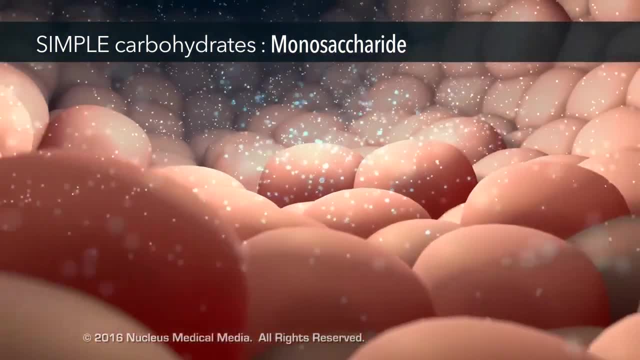 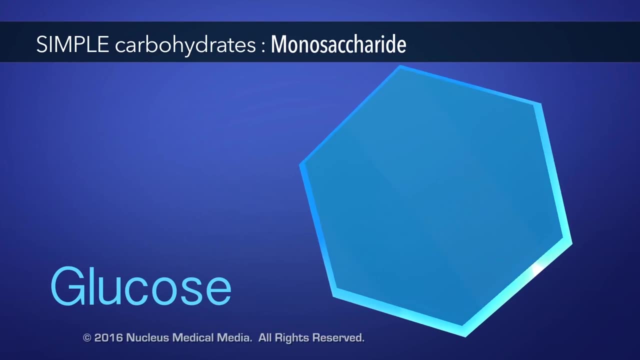 Simple sugars like glucose are the quickest form of energy because your cells can break them down easily. Words ending in "-ose" or "-ose" are typically sugars such as the monosaccharides, fructose, galactose and dextrose. 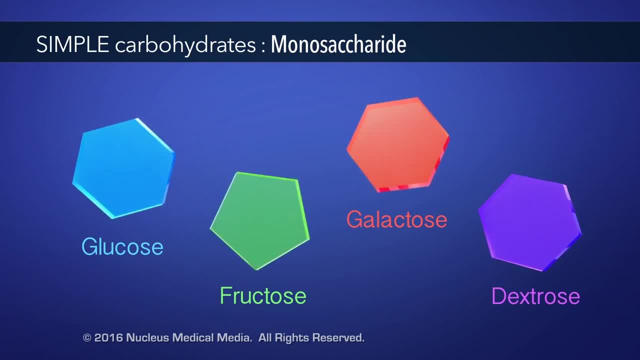 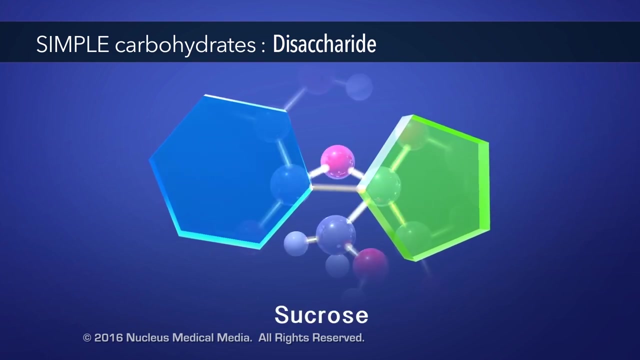 Like glucose, these monosaccharides are all simple sugars, because they are made up of a single sugar molecule. When glucose and fructose are chemically bonded together, we get a disaccharide called sucrose, commonly known as table sugar. 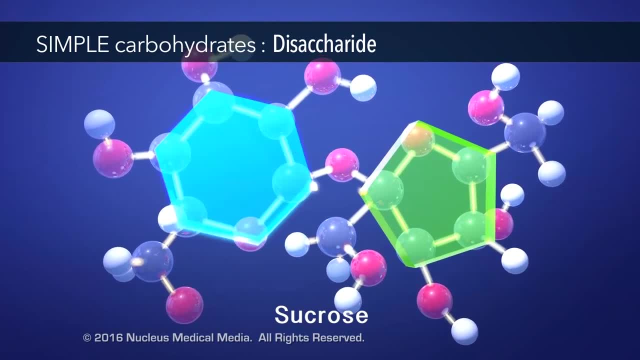 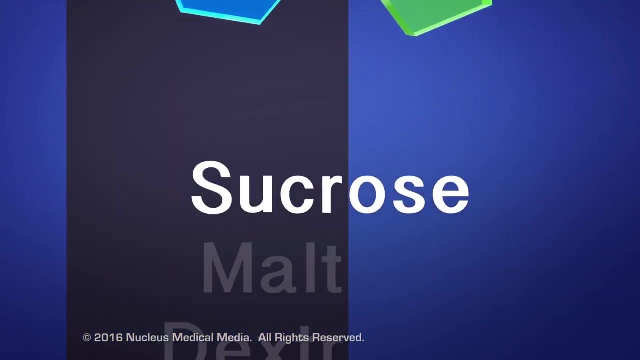 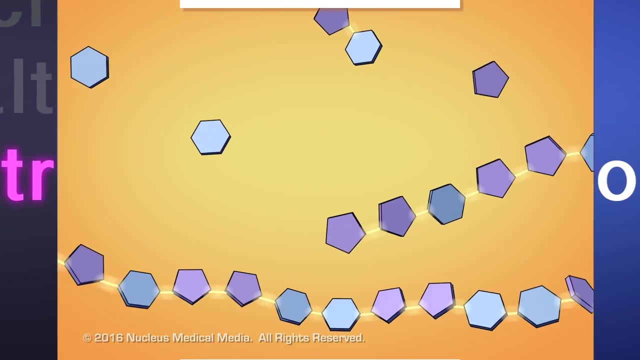 Sucrose is a disaccharide because it's made up of two monosaccharides. Like monosaccharides, disaccharides such as sucrose also end in "-ose" because they're sugar molecules. Now let's talk about complex carbohydrates. 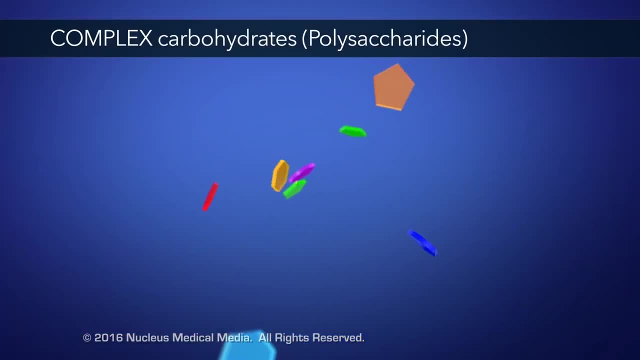 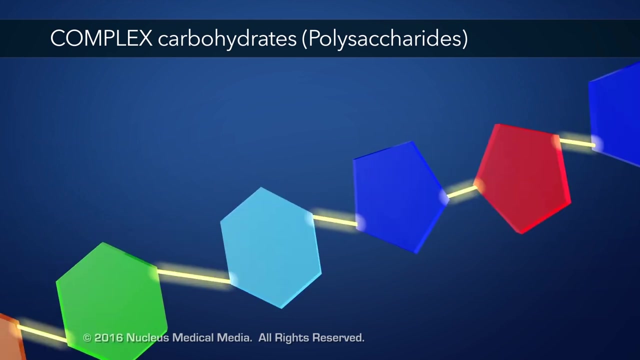 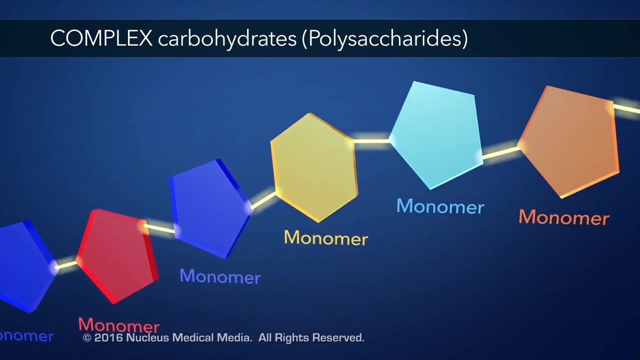 also known as polysaccharides. Polysaccharides are very long chains of multiple monosaccharides chemically bonded together. An entire polysaccharide is referred to as a polymer, while each individual monosaccharide in this long chain is referred to as a monomer. 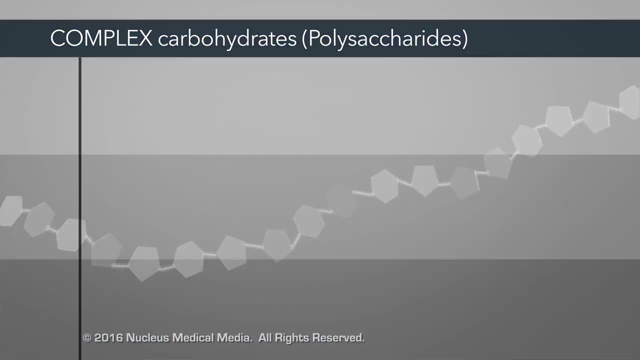 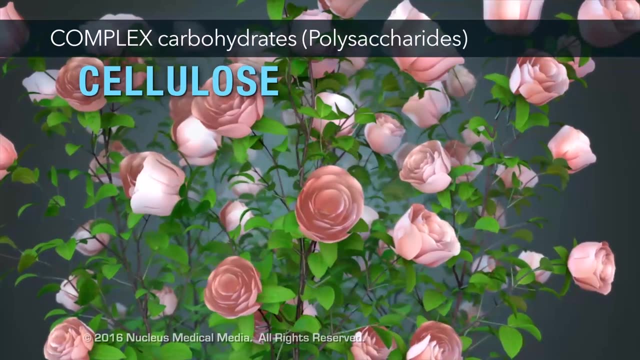 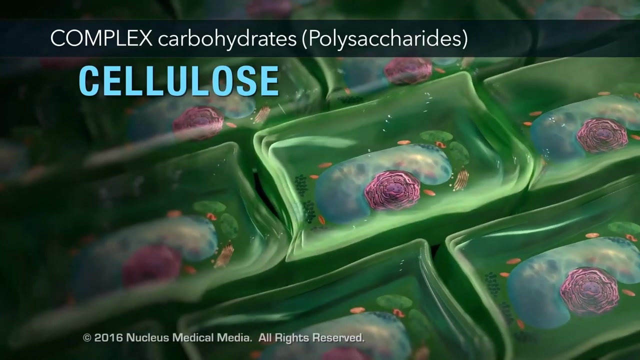 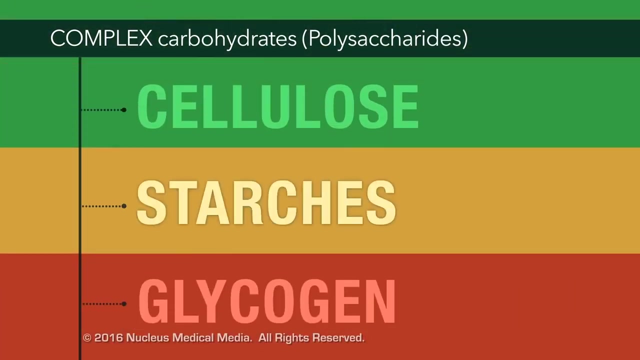 Examples of polysaccharides include cellulose starches and glycogen. Cellulose is found in all plants. It's a structural carbohydrate that is found in the cell wall of every plant. cell Starches are found in many of the foods we eat, such as potatoes and corn.